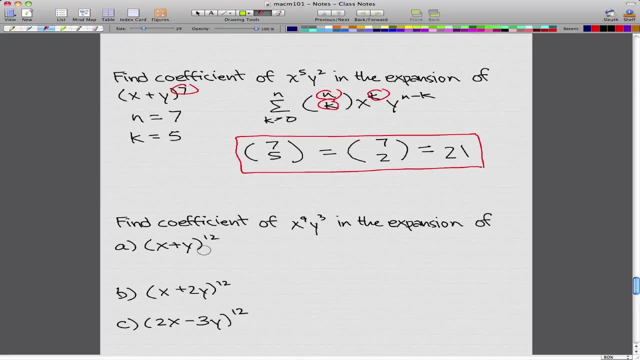 same as what we did in the last video. All we have to do here is, well, 12 is our n, and really we want x to the power of 9,, y to the power of 3, so k is pretty much our. 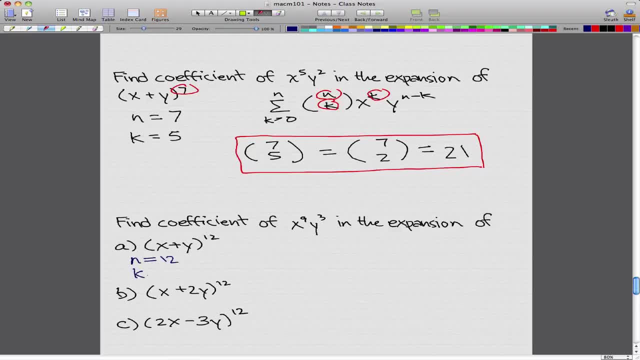 9.. So n is equal to 12,, k is equal to 9,. all we have to do: 12, choose 9, and that's our coefficient for x plus y to the power of 12.. And when we were looking for x to the power of 9,, y to the power of 3.. Now b is a little. 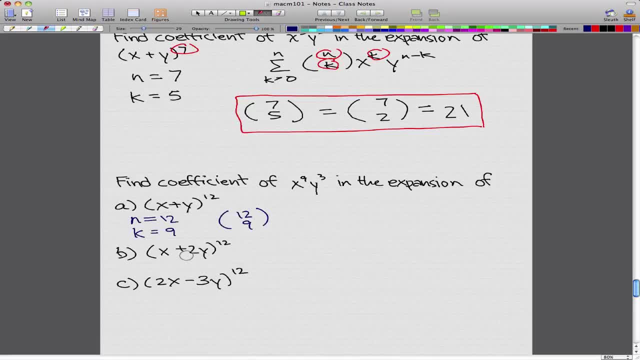 bit more tricky, but not that bad. What we want to do here is again: n would be 12, and k would be 9.. So our n minus k would be 3,, because 12 minus 9 is 3.. So what we? 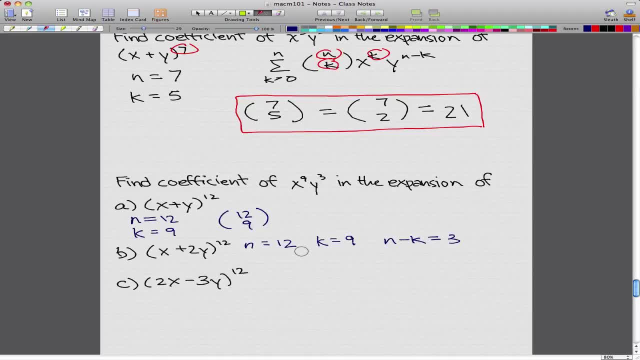 have to do is we go along and do the same thing- 12, choose 9,, nt- and then you'd think that would be our coefficient. but there's actually a little bit more work we have to do, Since there's. 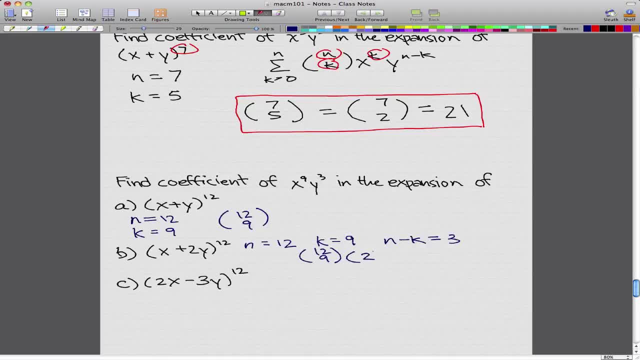 a 2 in front of this y, we actually have to take the 2, and we have to take it to the power of 3.. So the power of 3.. That will be our answer, Just because the 2 is in front. 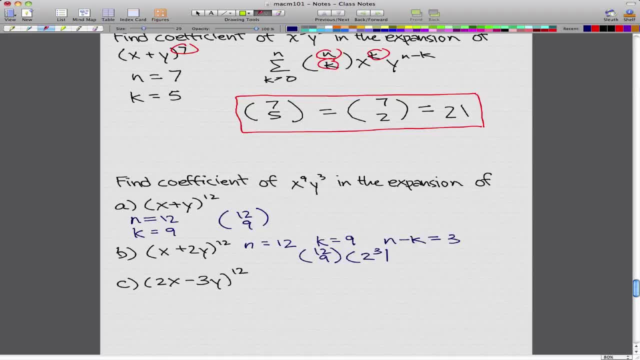 of that y, and we're looking for, uh, a coefficient, uh, that has y cubed in it. So that's as simple as that, And c is really a lot more tricky than what we just did. Well, again, it's not that bad What. 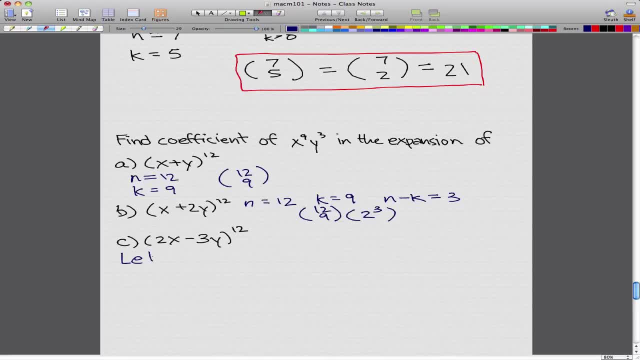 you want to do here is you want to have a couple of let statements. So let a equals 2x and let b equal negative 3y. So this whole thing now is going to be a little bit more difficult, Because this whole equation, uh, can be represented, This whole equation. 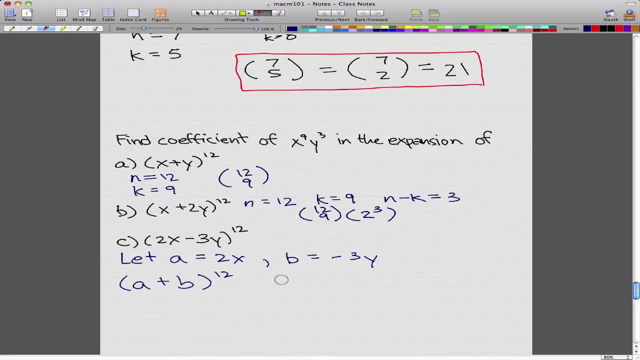 can now be simplified to a plus b to the power of 12.. And this x9 to x9y cubed, x9y cubed can also be simplified to a9b3.. Then all we have to do is we have to look for this, the. 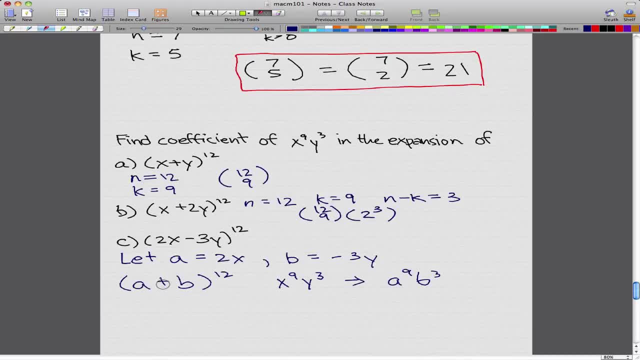 coefficient of this in con in the context of a. So this is the normal equation. So of a plus b to the power of 12. so let's just do that. so in our case, right now, n would be equal to 12, like always, and we're looking for, we're looking for n. 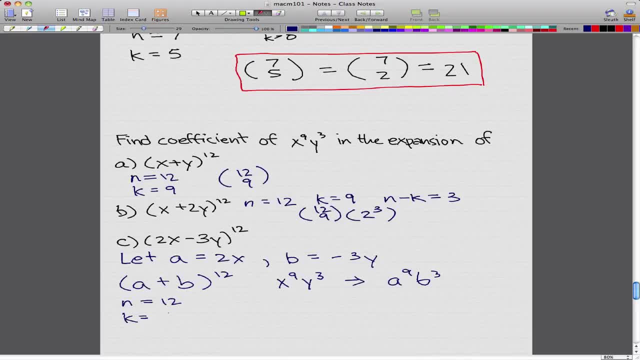 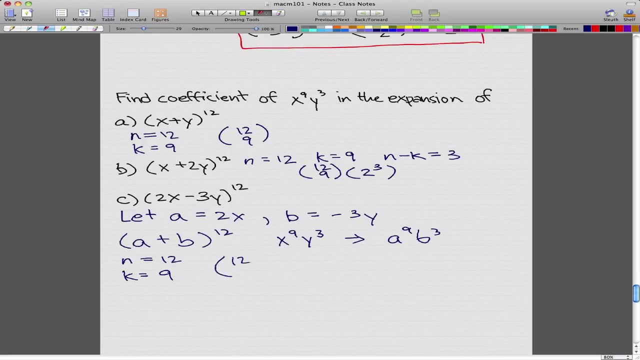 choose k, right? so then our k would be equal to 9 just like before. so nothing there has really changed. so doing that, we get 12, choose 9, but then we also have these A and B's. so, using that equation- where is that equation? using this: 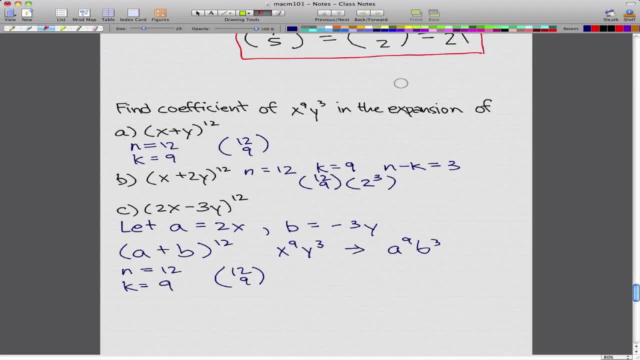 equation. we also have to factor in those A's and B's, so really, 12 choose 9 is really 12 choose 9. a, 9, B, 3. after this we want to turn the a's and b's back to their original X's and Y's. so what we have to do is: 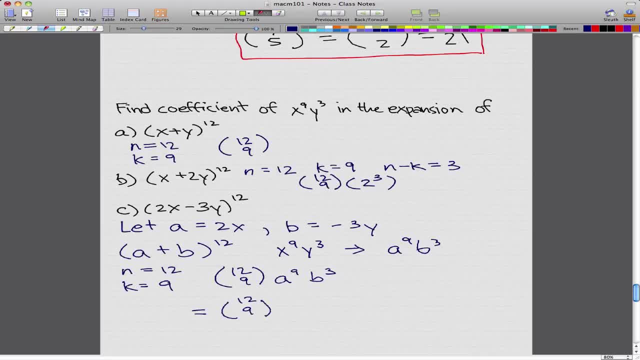 oh, oh oh. We pretty much we still have 12, choose 9,, but we turn a 9, and b 3 back to their original 2x's and 3y's. And that's pretty simple. We just take the a and just pop in a 2x to the power of 9.. 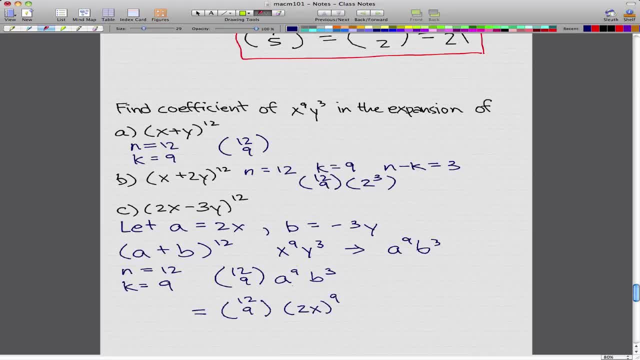 Because we have a let statement saying that a is equal to 2x. we can just substitute 2x for a And we do the same for b. So b would be minus 3. what Minus 3y to the power of 3.. 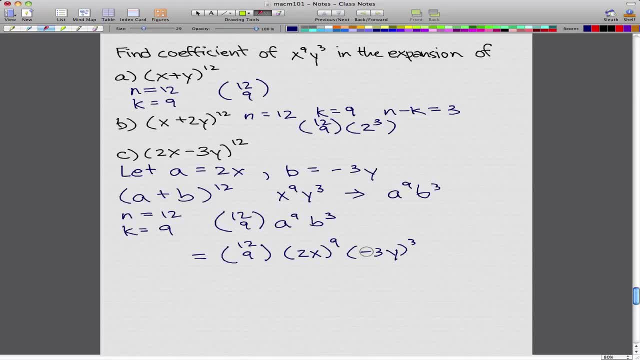 So what we can do now is we can just take out these 2 to the power of 9 and negative 3 to the power of 3 to get 12. choose 9,, 2 to the power of 9, and negative 3 to the power of 3,, x9,, y3. 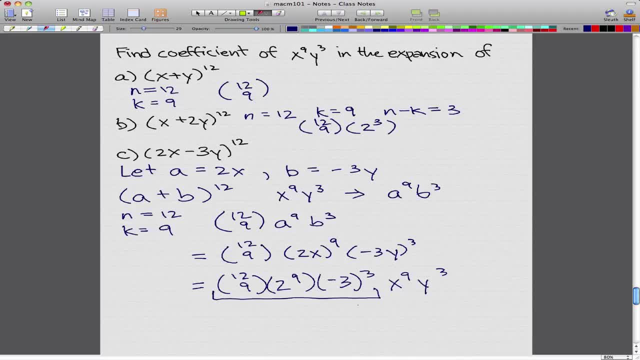 So this right here is our coefficient of x to the power of 9 and y3.. And really this substituting problem can also be used for b, but then I didn't use it for b because it's a better example with c, because we have both of them had to be substituted.